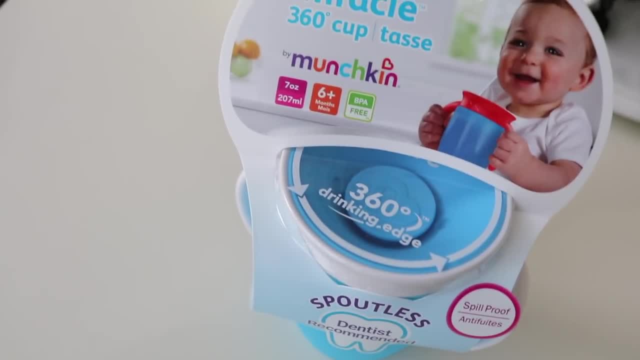 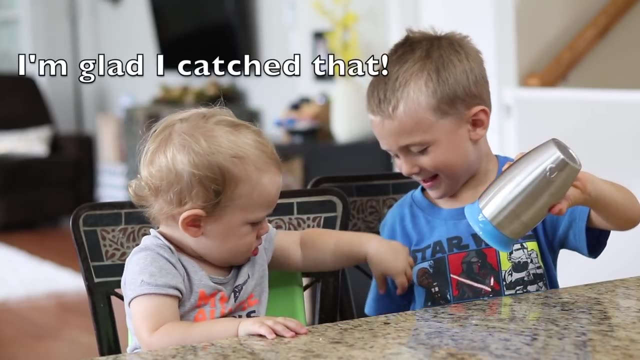 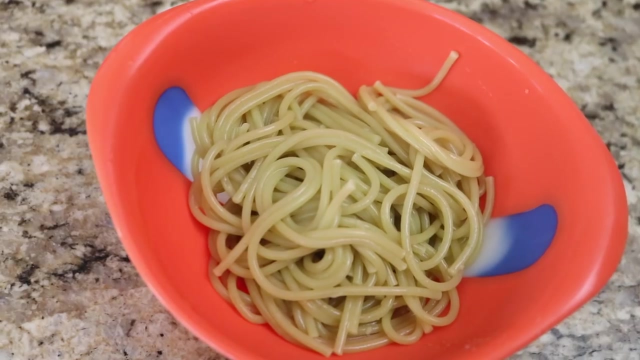 Leak proof cups are also great for teaching your kids to start drinking out of glasses, and mom doesn't have to worry about it getting all over the kitchen floor. Avoid meltdowns from food that's too hot by using utensils with white hot technology. 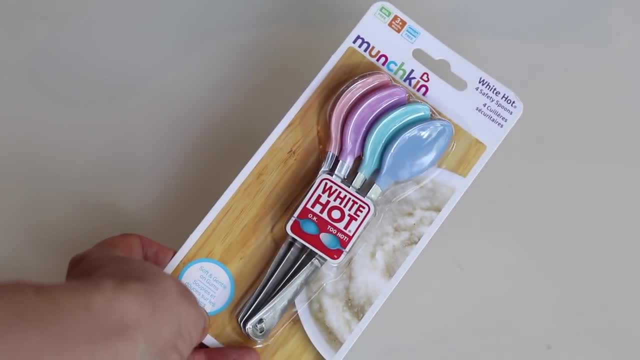 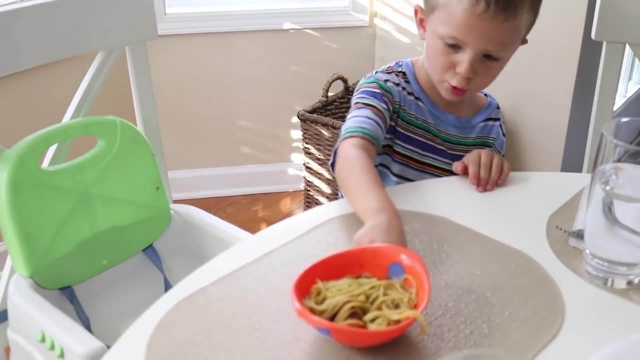 They turn white when the food is not ready to eat. If they're white, they're too hot. Is yours too hot? Yeah, see, And Baby Owen's is too hot too, And messes happen. So keep an OxiClean basket in your kitchen where you can throw clothes and bibs. 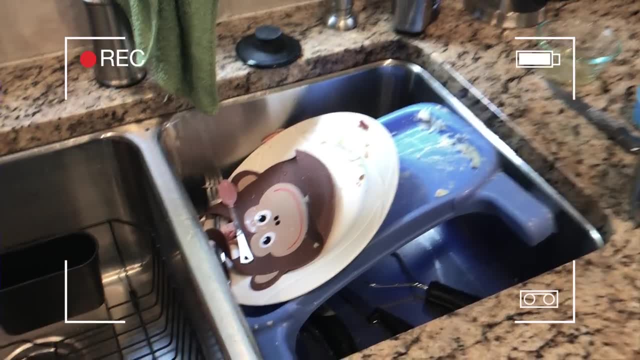 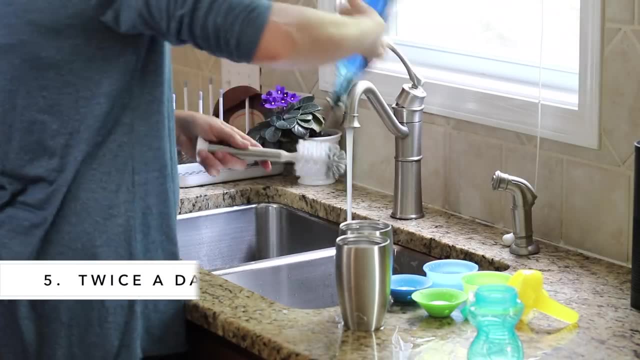 to get ready to soak and take out the stains. My house is not perfect. My kitchen is not perfect, So I aim to have a clean kitchen twice a day, morning and night. I work as I can to put things away and wash the dishes. I don't want to waste food. I don't want to waste food. I don't want to. 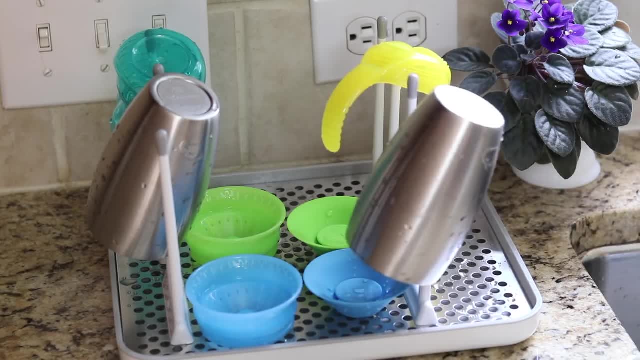 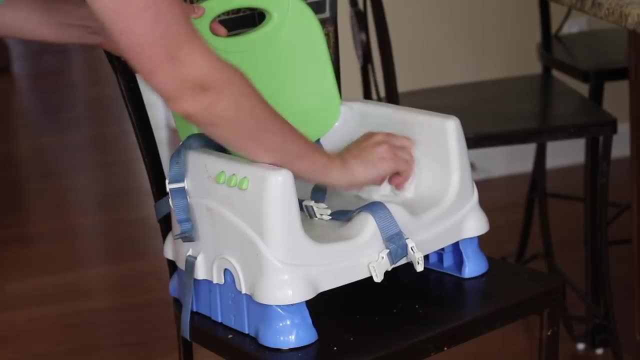 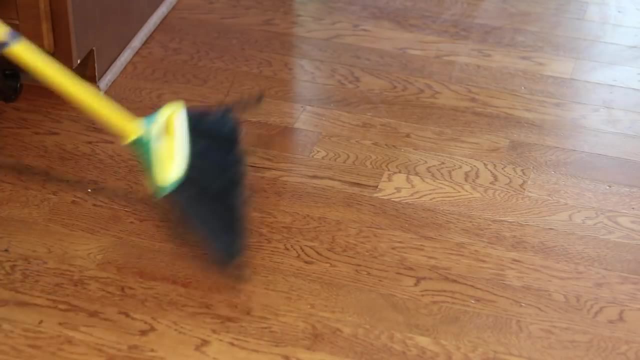 waste dishes And make less work. Assign each child a cup color and they use it all day long. I quickly wipe down and sweep between meals And if your kids have anything like rice or couscous or Play-Doh, wait for that to dry before sweeping it up. It will save you so much time in the long run. 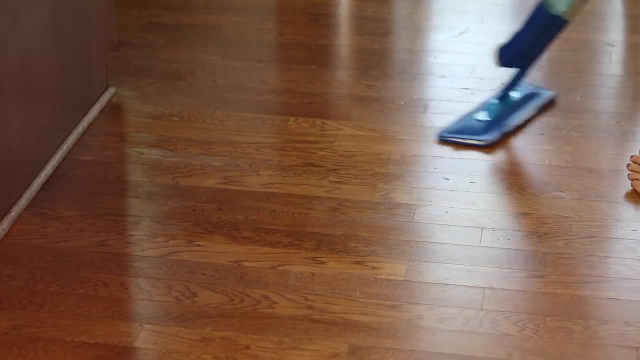 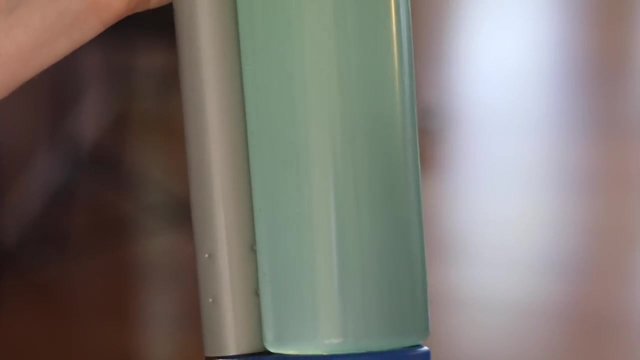 So I have a simple, ready to go mop with a removable Velcro pad. It's super easy to wipe down underneath of his high chair. I can just throw that pad in the wash when I'm done. Plus, all the solution is already prepared and ready to go. 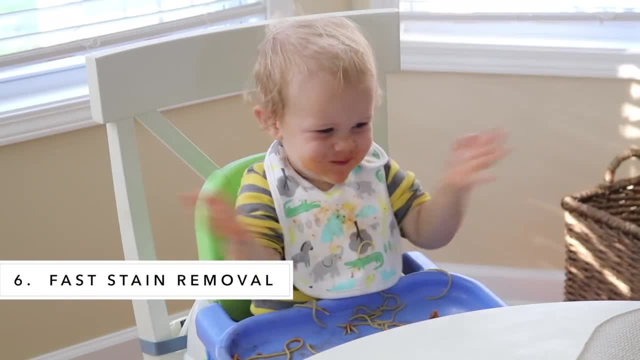 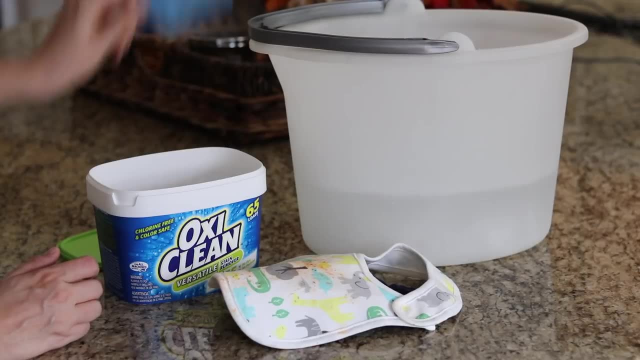 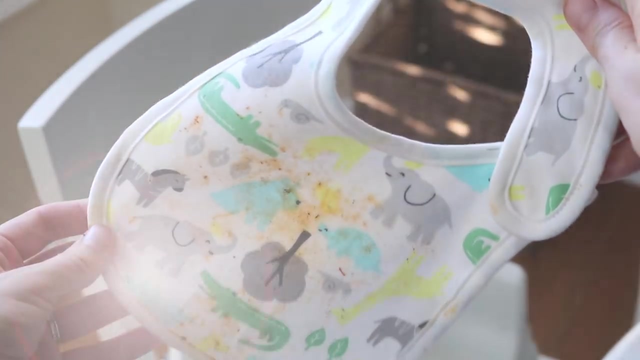 My next tip is to keep stain removal easy and fast On towels, high chair covers and bibs. I love using a stain remover that's dye-free. I can soak heavily soiled items or just add straight to my washing machine. It's zero extra work for me and money saved on otherwise ruined items. 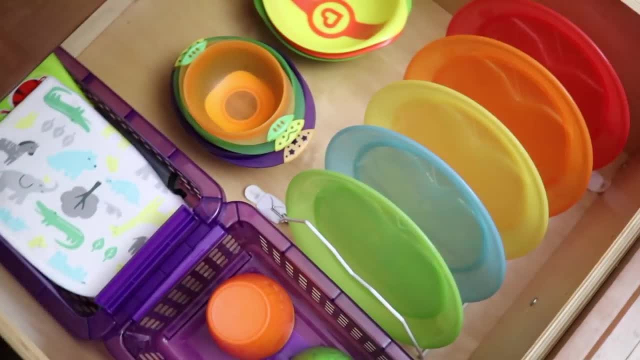 And that's it. I hope you enjoyed this video. If you did, make sure to hit the like button and subscribe to my channel. I'll see you in the next one. Bye. Let me know in the comments what do you do to keep your kitchen clean. 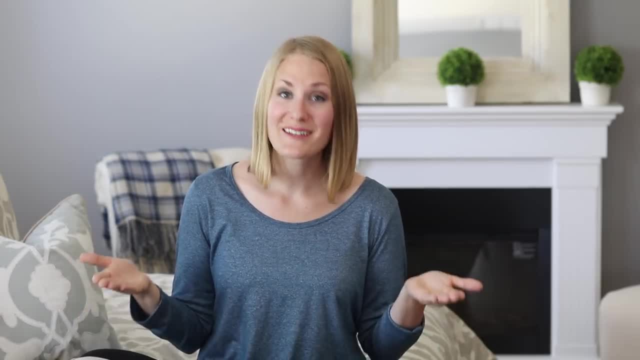 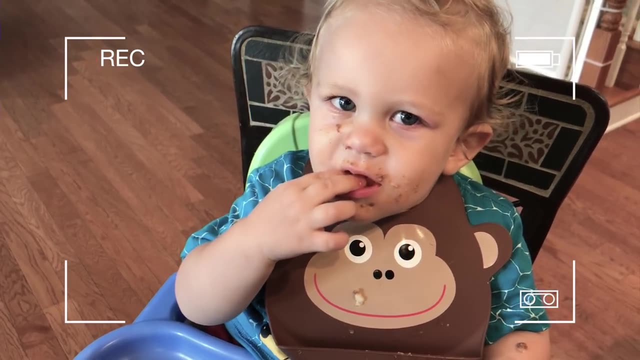 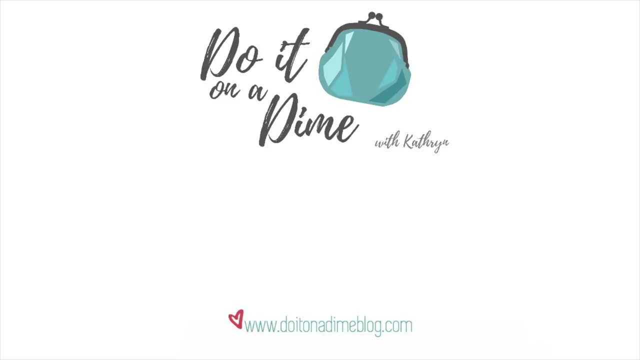 or what do you let slide? We're definitely not aiming for perfect at our house, just trying to make things a little bit easier. I'll see you guys in the next video. Bye, What do you think of it. Let me know in the comments. what do you think of it?